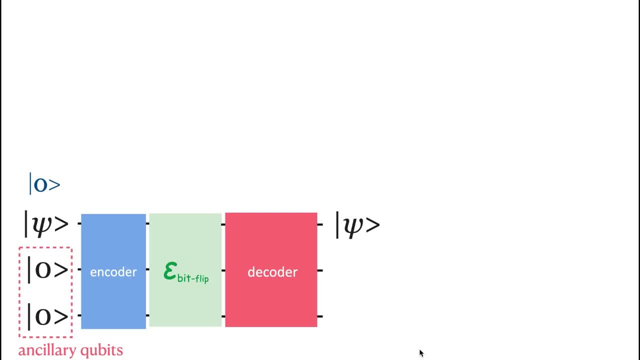 carrying the information will be the same as the input. So when we send the information from the input, the information will be encoded into a greater number of qubits. In this case, the qubit with the information state zero will be encoded with two ancillary qubits. 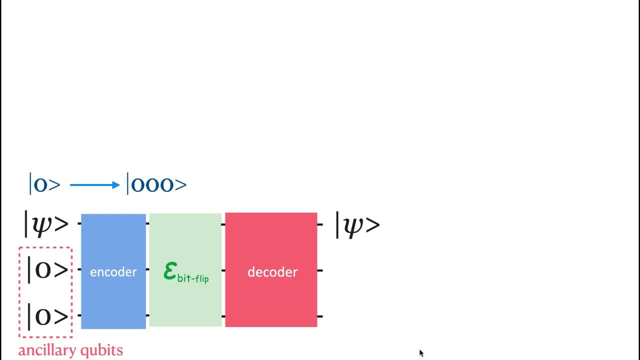 After the encoding process, the input becomes state zero, zero, zero, And there's a chance that while the information is transmitted from the input to the output, the qubits might be flipped. If we look into the encoder, let's say that the main qubit state was zero. 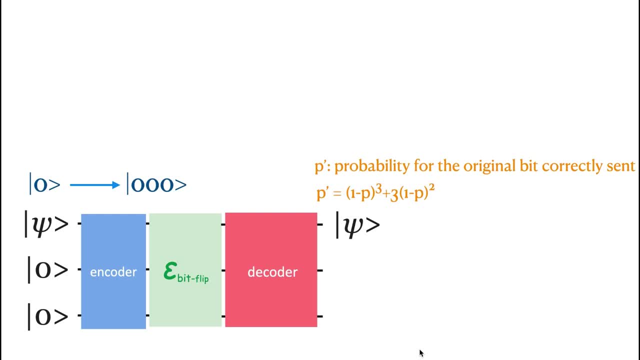 We can see that the main qubit state was zero. So we can see that the encoder will be passed to the decoder and the decoder will then correct the information And at the output we can get the information with the probability of p. If we look into the encoder, let's say that the main qubit state was zero. 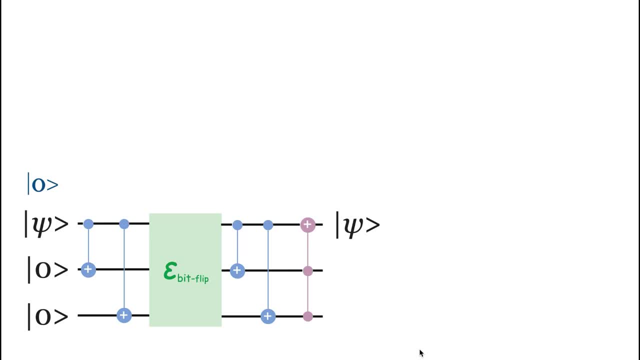 Two CNOT gates will be applied to the ancillary qubits, which will leave them unchanged, since the main qubit state was zero. There are two CNOT gates connected to the target state and the control state. The first two qubits will be encoded with one CNOT gate, And the third qubit will then also be. 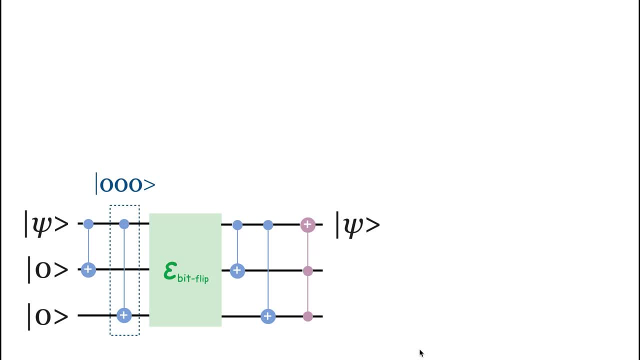 encoded. so the three qubits will be encoded into a greater number of qubits. The second qubit will be encoded by the two CNOT gates together. to add the two CNOT gates, The second qubit will be encoded with two CNOT gates. 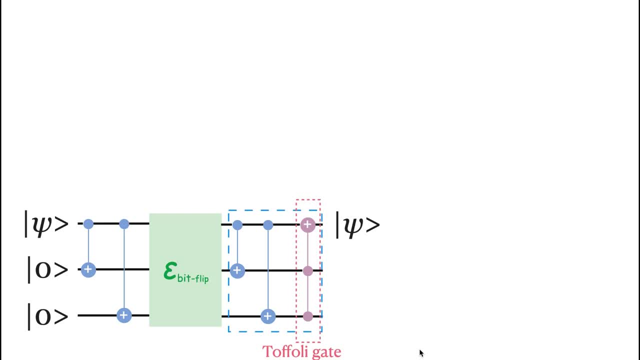 After passing through the bit flip simulation and the decoder in order to correct the bit flip, the CNOT gates are applied to the ancillary qubits After passing through the bit flip simulation and the decoder, and then a TOEFLIT gate is applied to the first qubit, which will correct its. 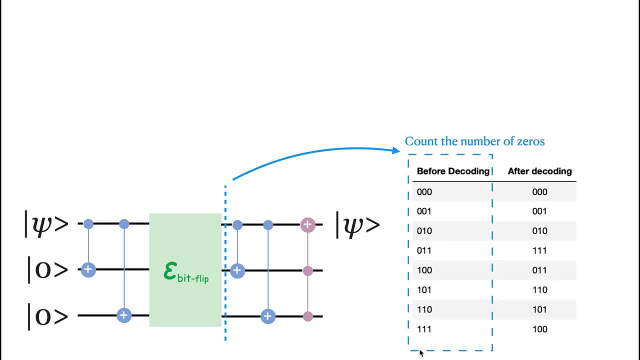 state. The decoder works like a counter, counting the number of the zeros of the output and then decides what the information of the first qubit was carrying. If at the output state there are more zeros than ones, then the decoder will decode the information to be zero state, which means that the first qubit